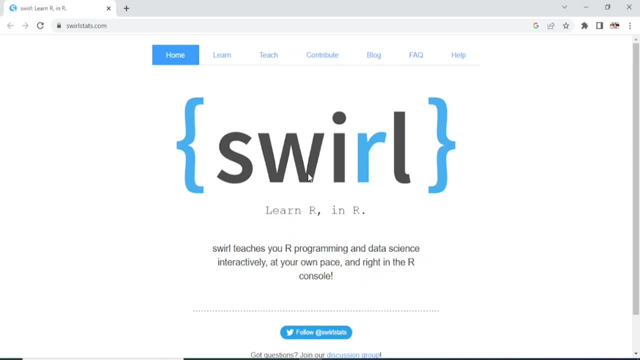 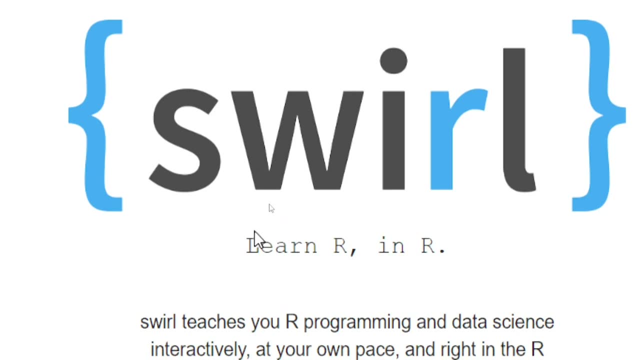 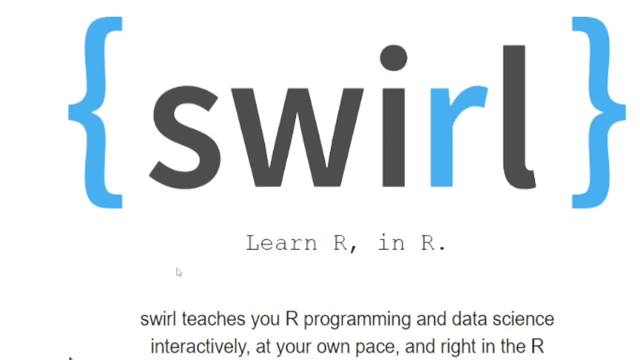 Hello everyone and welcome back to my channel. This video is going to be very exciting, as in this video, I will talk about a very special package known as swirl. This package can be used to learn R within R. Swirl teaches you R programming and data science interactively, at your own pace and right in the R console. So you don't need to go anywhere to learn R. 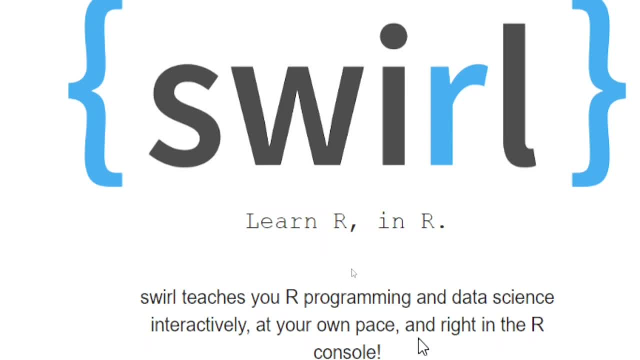 You can learn R programming at any time in your R console, So this package is really really interesting and learning R through this package is really a fun. I'm sure you will definitely enjoy learning R through this package. So, without wasting our time, let's start learning R through this swirl package. 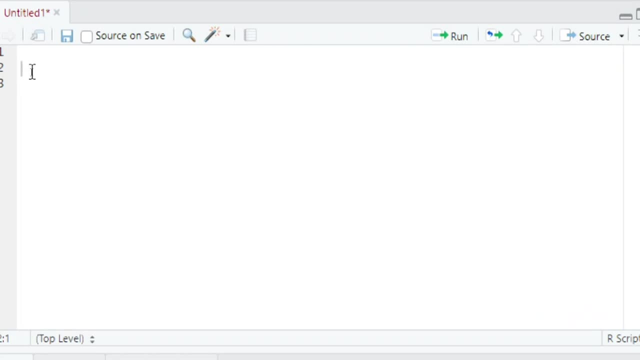 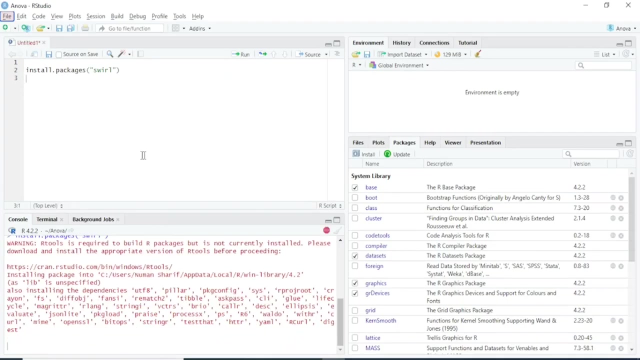 Okay, first you have to install a swirl package. So to install a swirl package. you have to install a swirl package. So to install a swirl package. type installpackages- quotation mark and press ctrl enter to run this function. Okay, it might take some time to install this package. 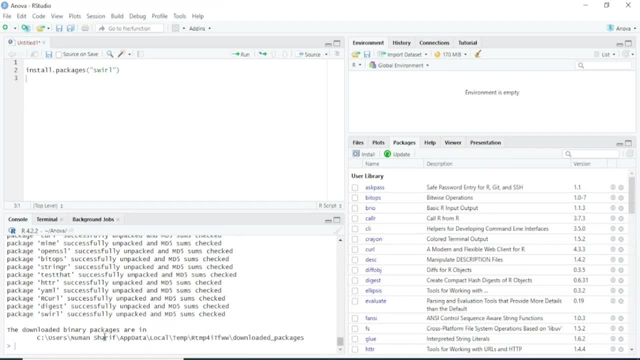 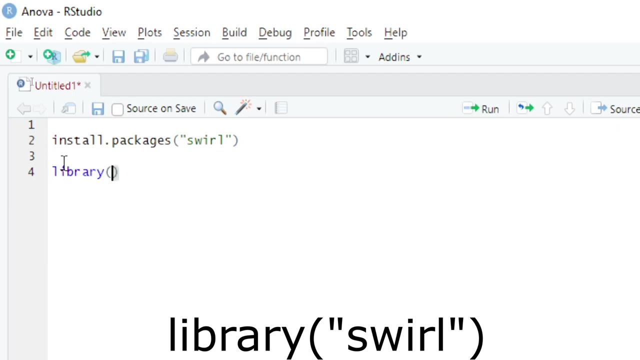 Okay, so now you can see here: swirl package has been successfully installed. Okay, to start learning through this package, you have to load this package. To load a package you have to type library, then write the name of the package which you want to load and press ctrl enter. 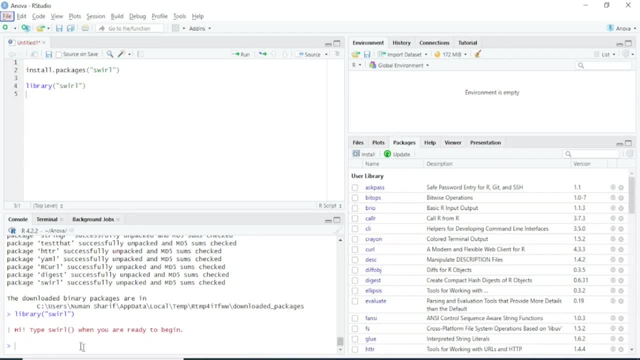 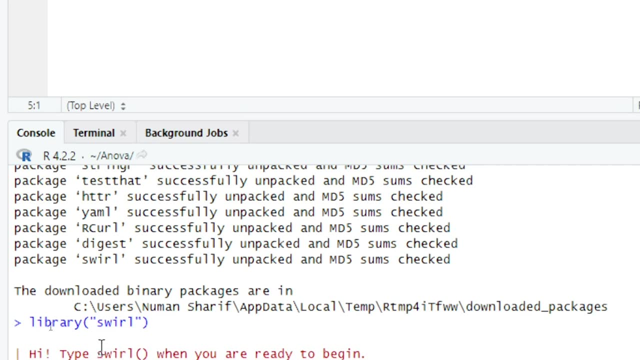 Okay, now you can see the swirl package has been loaded now. Okay, now swirl has been loaded, So we will use console to type different codes and will not type codes in script file, because it's easy to interact with swirl package through console. 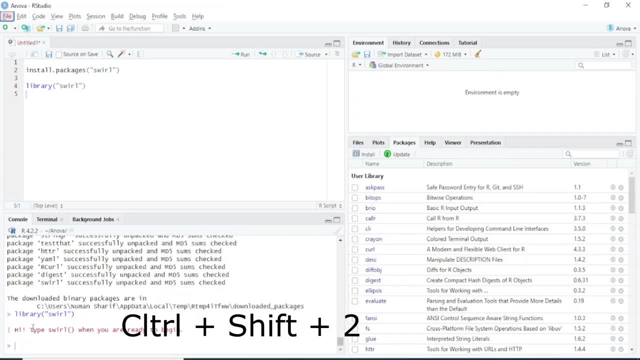 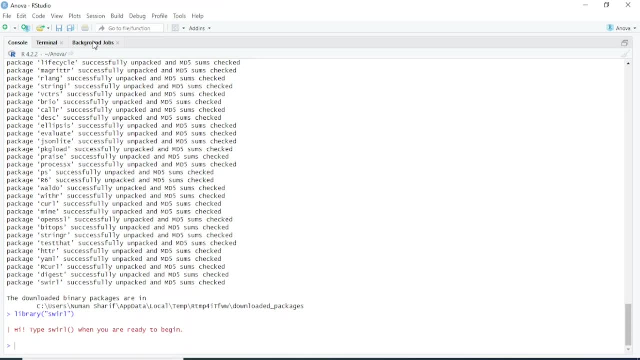 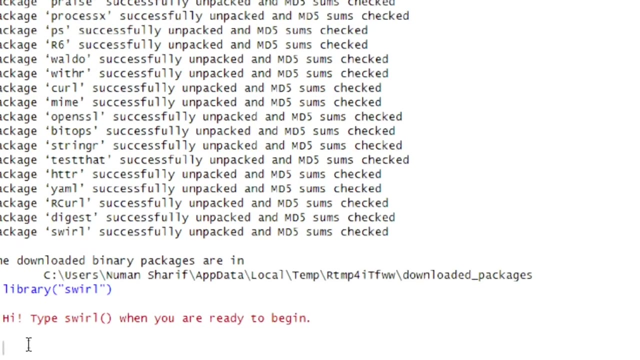 So I will press ctrl shift 2 to directly zoom into R console. Okay, So now you can see we are only seeing here R console, and all the other things have been disappeared. package has been loaded now what you have to do you have. so it's saying hi, type, swirl when you 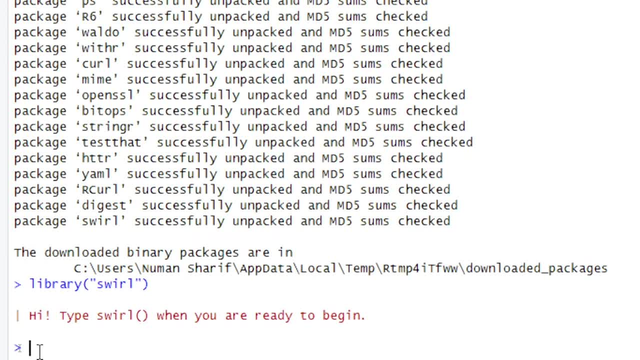 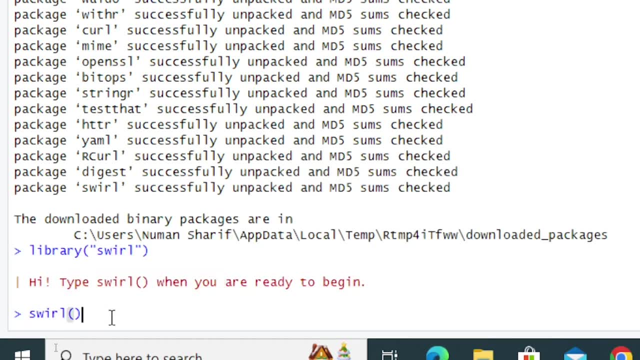 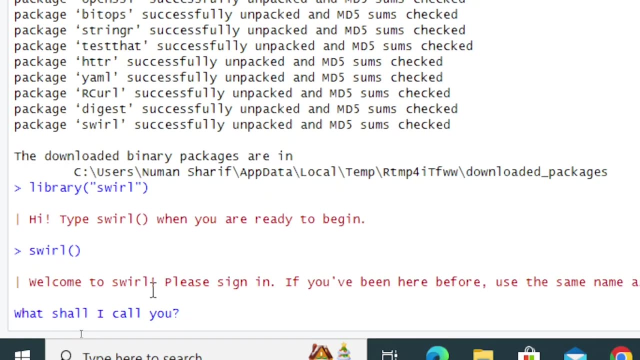 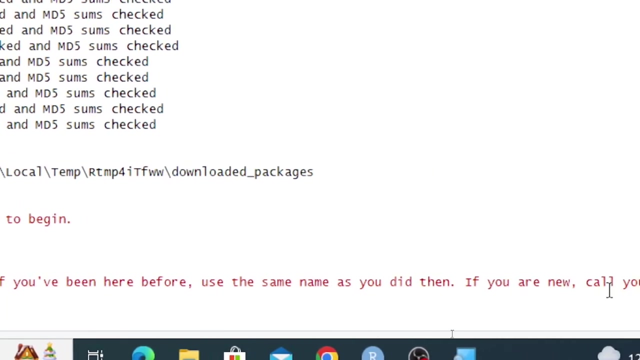 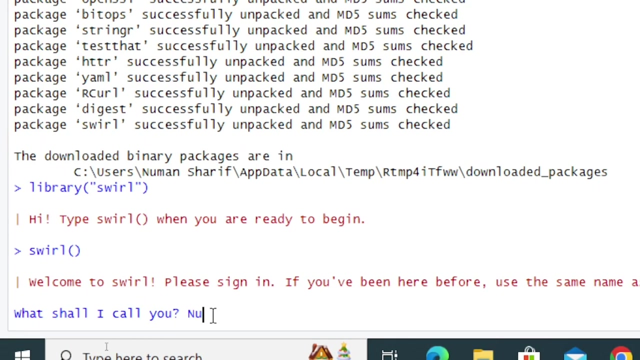 are ready to begin. okay, so let's type uh, swirl- open parenthesis, close parenthesis and press enter. okay, so welcome to swirl. please sign in. if you have been here before, use the same name as you did. if you are new, call yourself something. okay, let's call myself numan. okay, thanks, numan, let's. 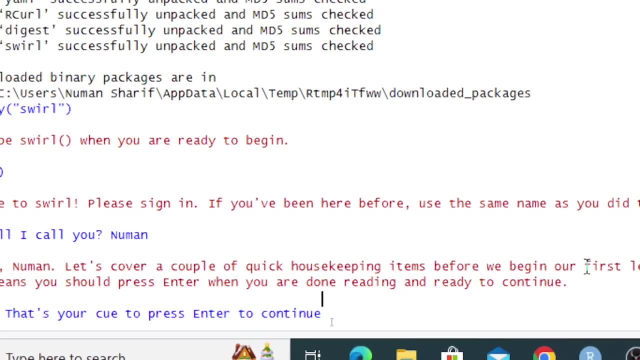 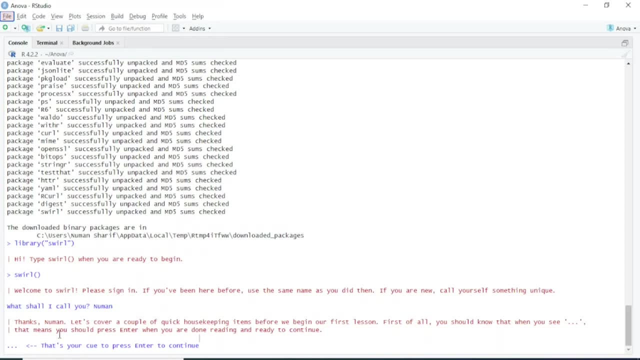 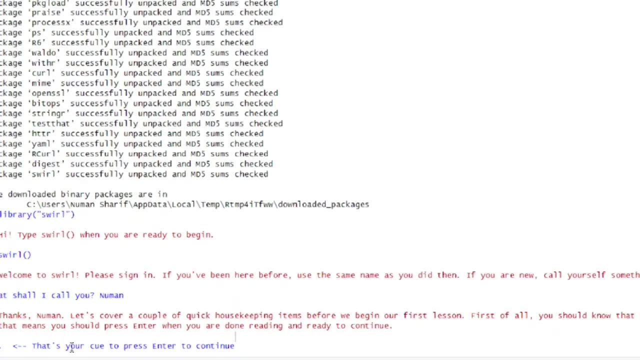 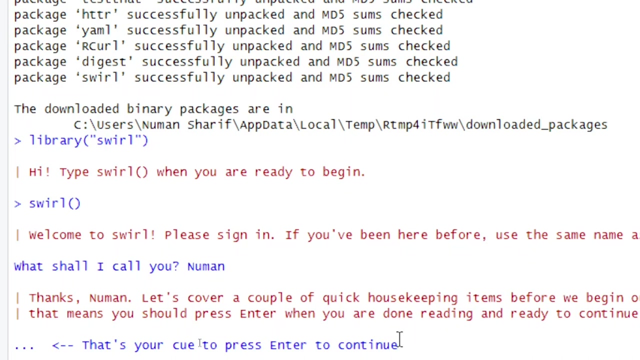 cover a couple of quick housekeeping items before we begin our first lesson. first of all, you should know when you see dot dot dot, that means you should press enter when you are done reading and ready to continue. okay, so here you see dot dot dot. that's your cue to press enter to continue. so let's press enter. 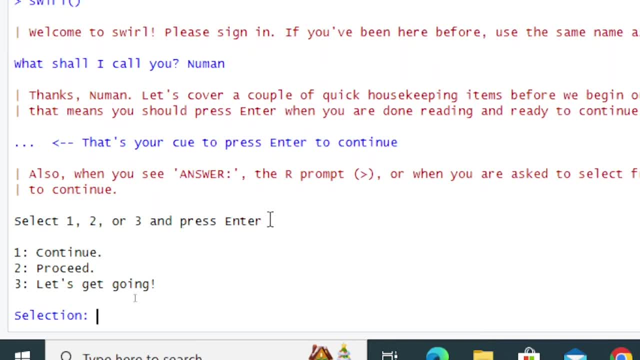 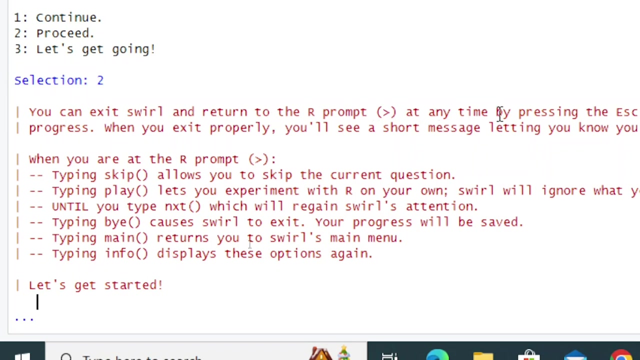 okay. so now it's asking: select one, two or three and press enter. one means one for continue to proceed. three let's get going, okay. r of these three functions means the same thing, so let's press two, okay, okay. you can exit swirl and return to our prompt at any time by pressing the escape key. 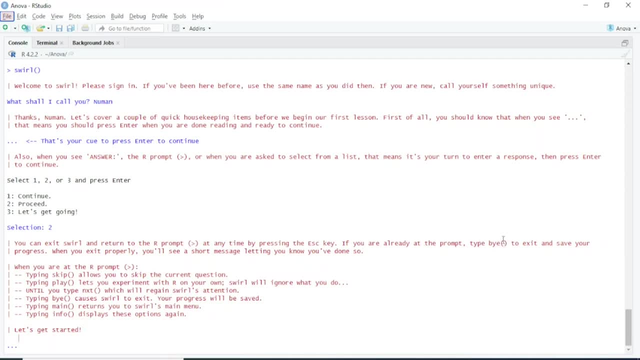 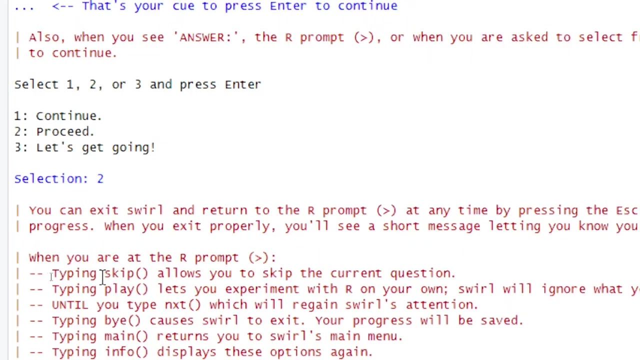 if you're ready at the form type by open parenthesis, close parenthesis, to exit and save your progress. when you exit properly, you will see a short message letting you know you have done so. let's get started. okay, so here are different keys: which, uh, which uh, for different things: typing: 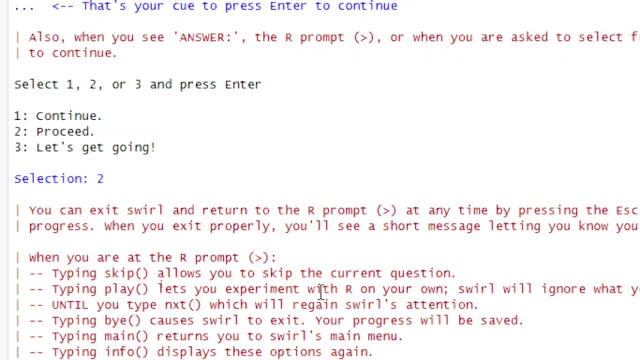 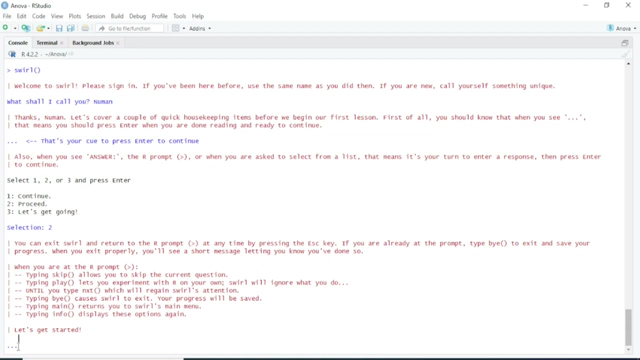 skip allows you to skip in the current question. typing play lets you experiment with r on your own and typing next, and typing by little causes swirl to exit, and so on. you can read, uh, the detail of all of these keys. so let's get started. you are seeing dot dot dot. it means we have to press uh enter to continue. so i pressed enter to 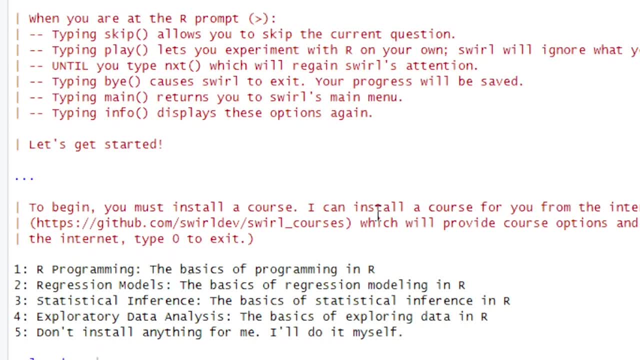 continue. okay, to begin, you must install a course. i can, i can install a course from you, from the internet, okay, so, uh, there are different courses which you can install, and for your practice, okay, the first course is r programming, the basics of r programming in r. the second one, 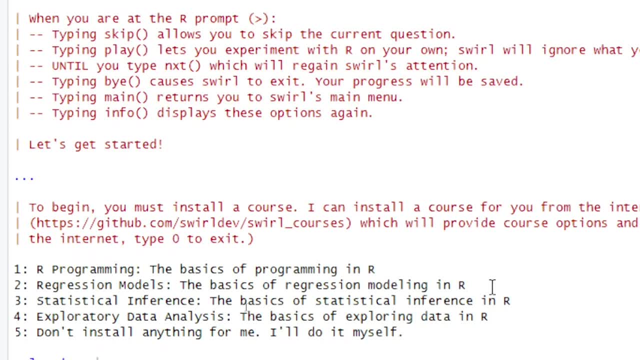 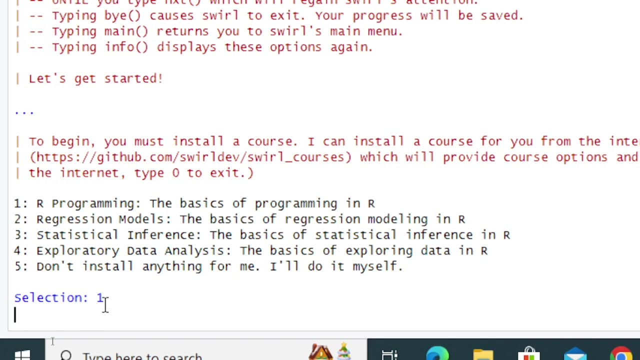 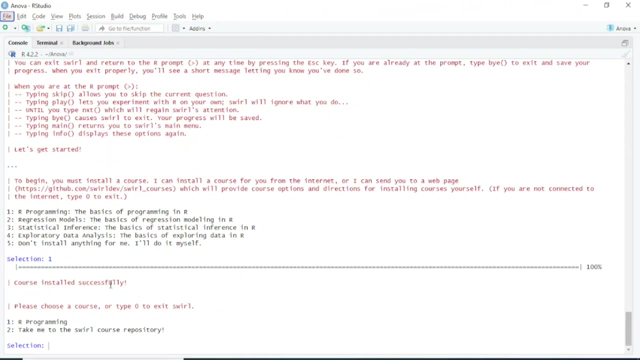 is regression models, the basic of regression modeling in r. so i will select one. i want to learn r programming and the basics of r programming, okay, so i pressed one and enter. okay, now it will install the course and you can see. course has been successfully installed now. okay, now it is asking: 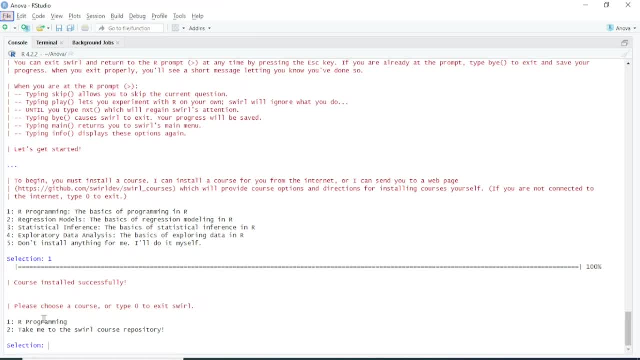 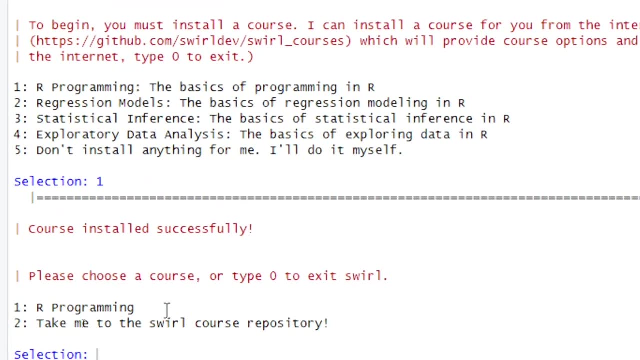 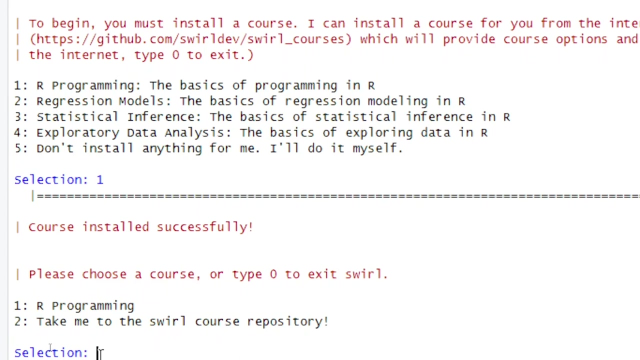 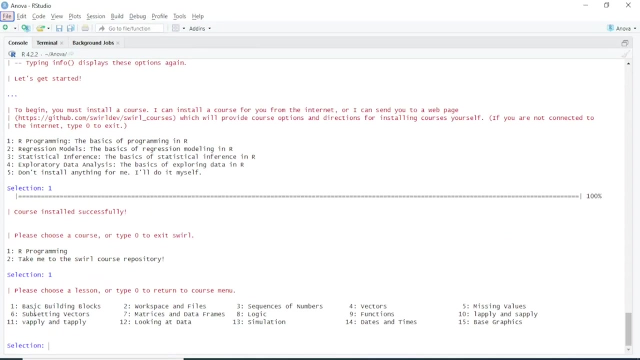 a course or type 0 to exit swirl. okay, so we we will choose a course. okay, it is asking one for r programming and two: take me to swirl course repository. okay, so i will type here one for r programming, okay, and press enter okay. now again it is asking: please choose a lesson or type 0 to return. 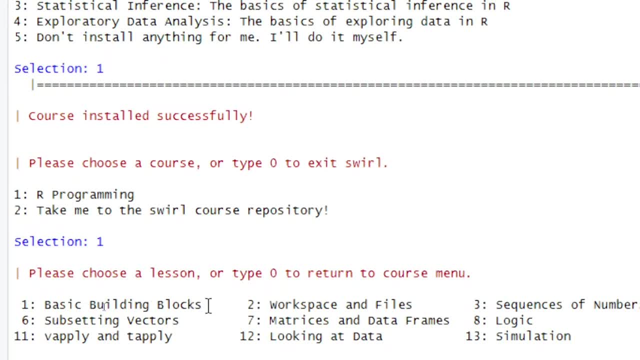 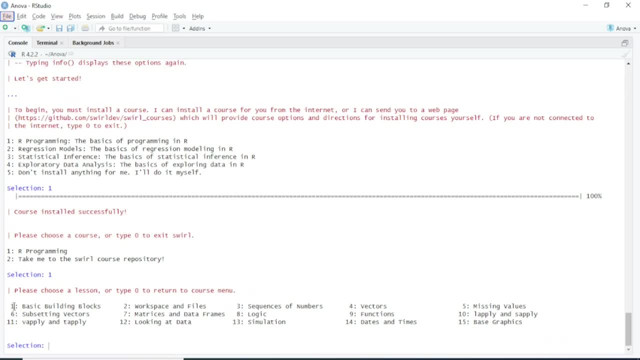 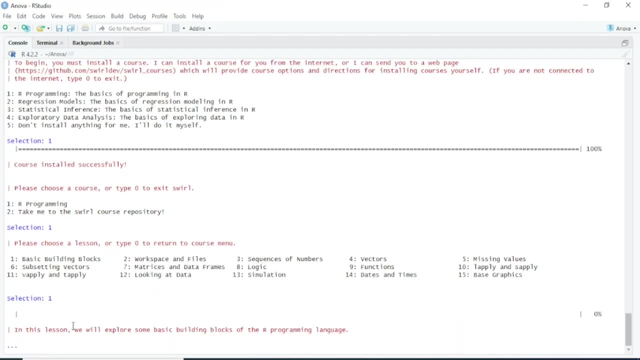 here. the first lesson is basic building blocks. the second one is workspace or files. so i will go for first lecture. okay, select one and press enter. in this lesson we will explore some basic building blocks of our programming language. okay, and here you are seeing dot, dot dot. it means we have to. 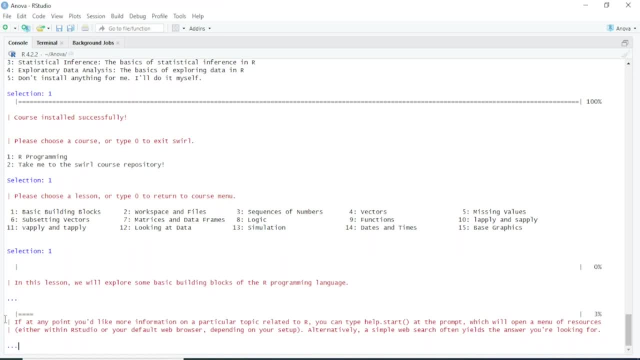 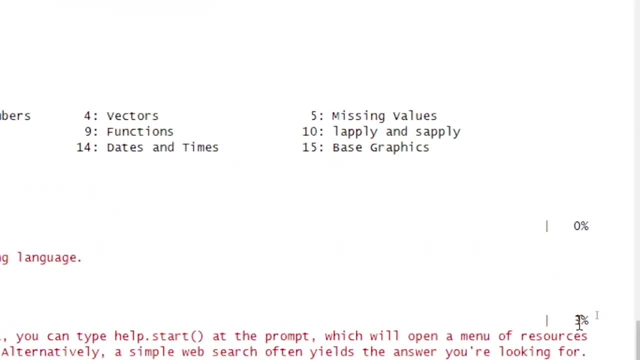 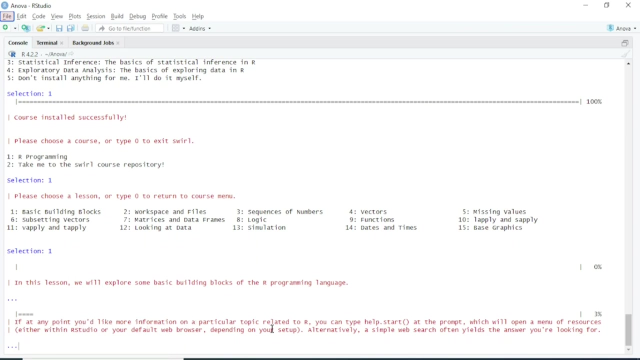 select a lesson or type 0 to exit swirl. okay, so i will click on it and press enter. okay, so i have pressed enter. you can also see here the progress through this line as we have completed this lesson: three percent okay. so if any point you would like more information on particular topic related to r, 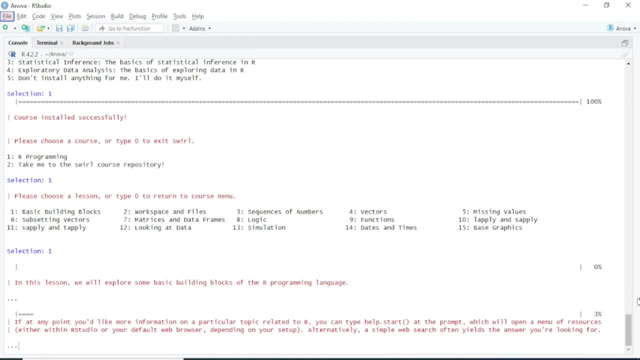 you can type help, dot, start at the prompt, which will open a menu of resources, your default web browser, depending upon your setup. you can read all of the instruction and you can play with it. okay, so here you are seeing dot dot dot. it means we have to press enter. so now you can. 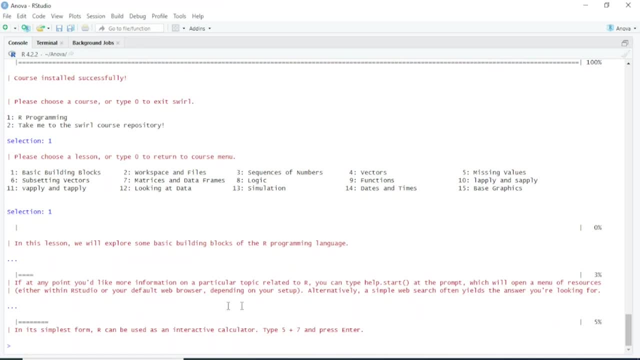 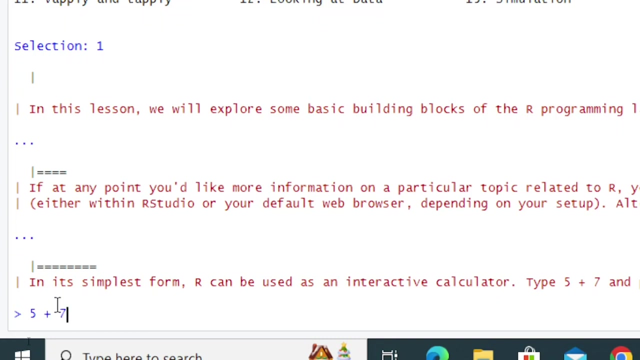 see the five percent of lesson is completed. in its simplest form, r can be used as an interactive calculator. okay, so first we will use r as an interactive calculator. so it is asking: type 5 plus 7 and press enter. so here i will type 5 plus 7 and press enter. so 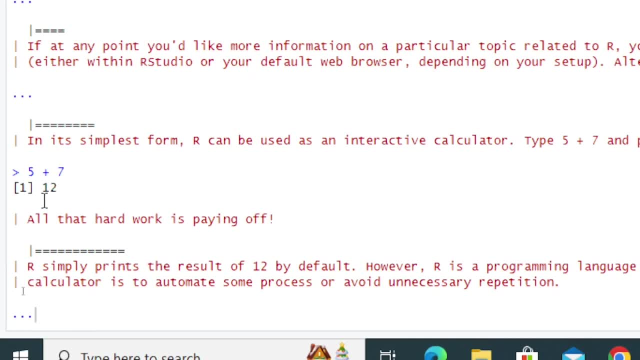 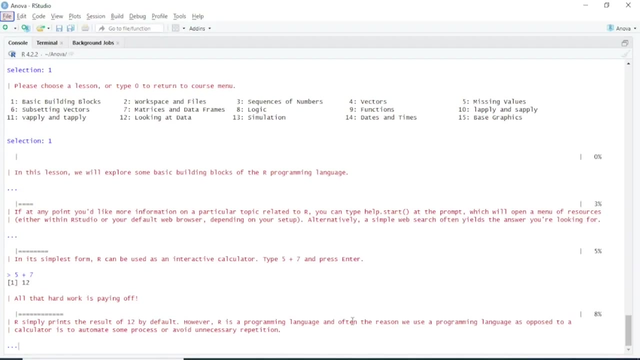 okay, so here you can see the result: 12. all that work is paying off, so, as i said earlier, it's really fun. so r simply prints the results of 12 by default. however, r is just a general calculator which is usually used for programming language and and often the reason. 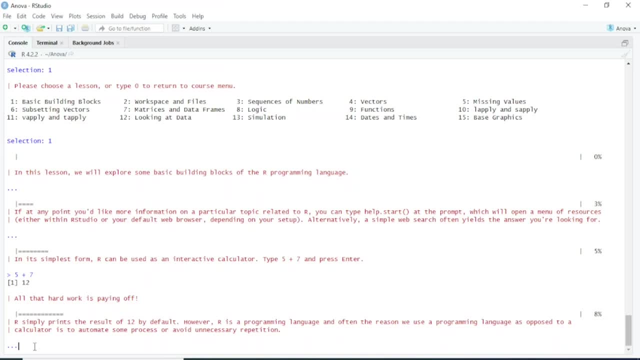 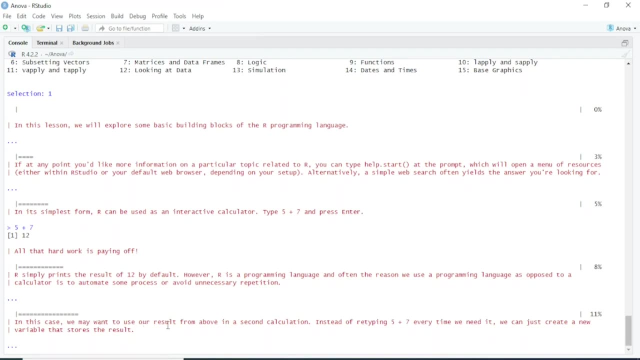 we use a programming language is opposed to as calculator. okay, again, you are seeing dot dot dot. it means we have to press enter again. so i again press enter. in this case we may want to use our result from above in second calculation instead of pre-typing 5 plus 7 every time we need it. we can. 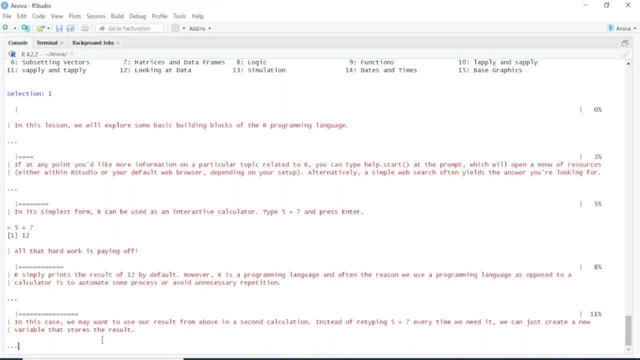 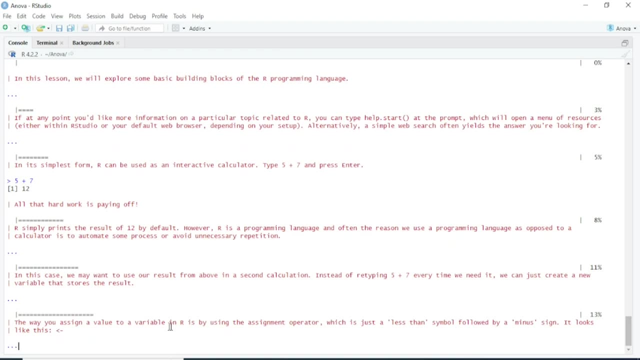 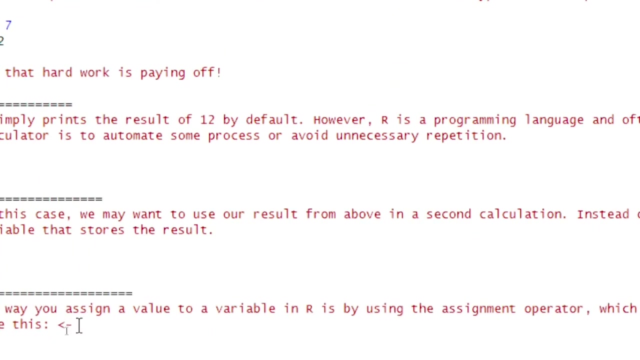 create a new variable that stores the wizard. okay, dot, dot, dot enter. the way you assign a value to a variable in R is by using the assignment operator, which is just less than some, which is just less than symbol, followed by a minus sign. it looks like. it looks like this okay. okay again, I have to press enter. okay. 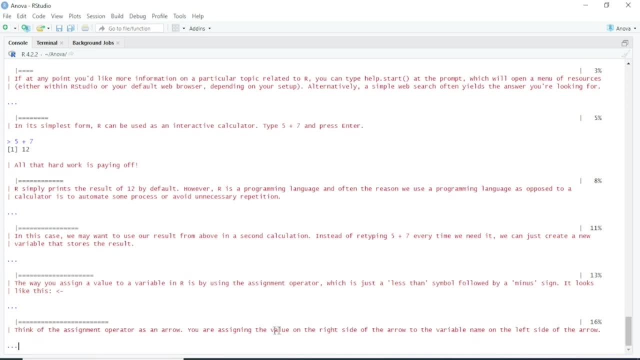 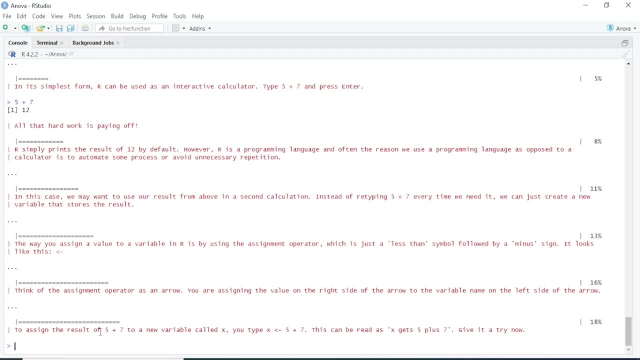 think of the assignment operator as an arrow. okay, you can read all of these details and again press ENTER to assign the results of 5 plus 7 to a new variable called X. type X. assignment operator: 5 plus 7. okay, so here, right, we will write X.